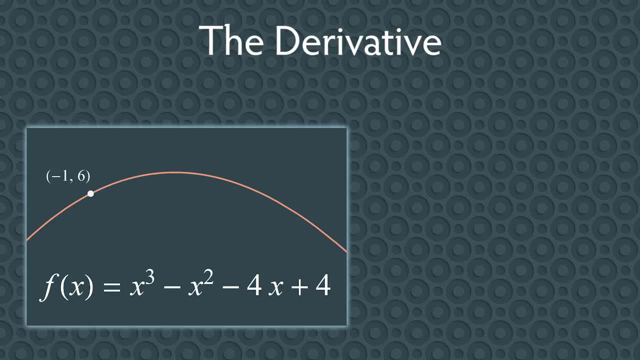 Here's the idea. pick a second point nearby. How about the point negative 0.8, 6.048.. Next, draw a line through these two points. The slope of this line is a good approximation for the steepness of the curve. at the point negative 1: 6.. 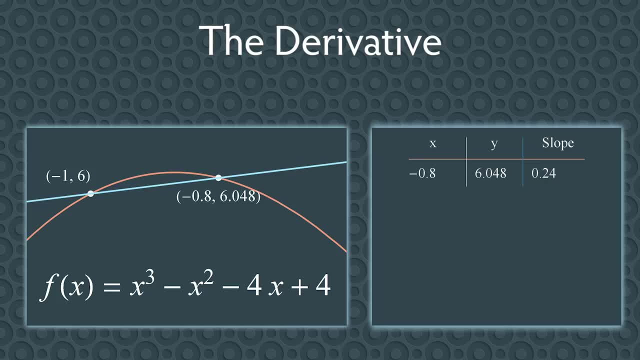 If you compute the slope, you get 0.24.. This is a good approximation, but we can do better. What if we pick a different point that's even closer? How about negative 0.9, 6.061.. If you compute the slope of the line through this point at negative one six, you get 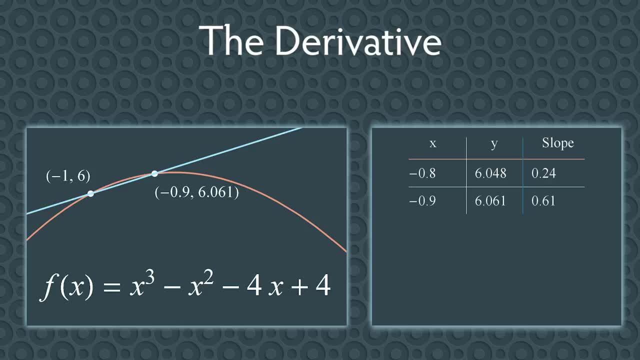 0.61.. If you keep picking closer and closer points and computing the slopes of the lines, you'll get a sequence of slopes which are getting closer and closer to some number. The lines are getting closer and closer to the tangent line and the slopes are approaching one. 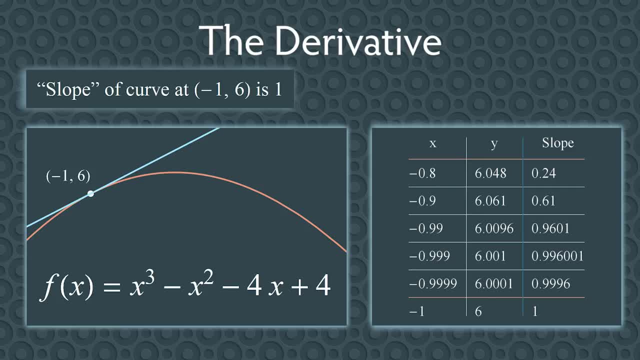 So we say the slope of the curve at the point negative one six is one. We call this number the derivative of f of x at the point where x equals negative one. This is the slope of the tangent line through the point negative one six. Luckily you won't have to do this every time you want to. 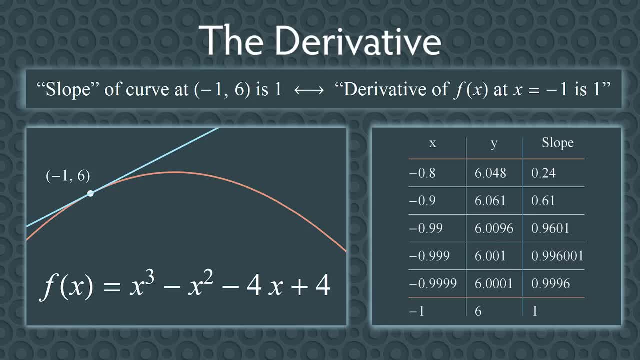 measure the rate of change at a point. In calculus you'll learn how to find a function which will give you the slope of any tangent line to the graph. This function is also called the derivative, So we say the slope of the curve at the point negative one. six is one. We call this number the. 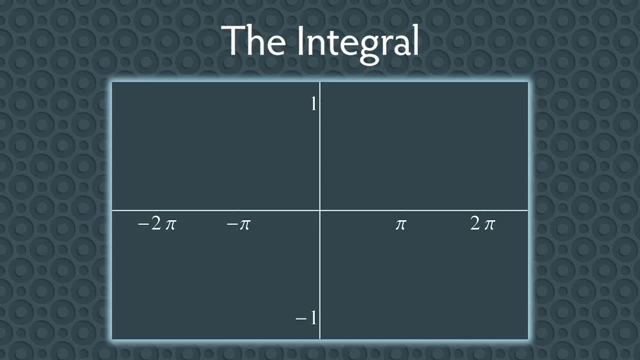 derivative. Next, let's take a look at the integral. This is the tool that lets you find areas under curves. As an example, let's look at the function g of x equals sine x. What if we wanted to find the area under this curve between x equals zero and x equals pi? How would 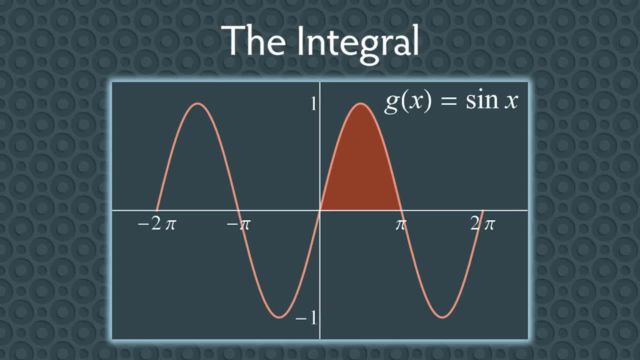 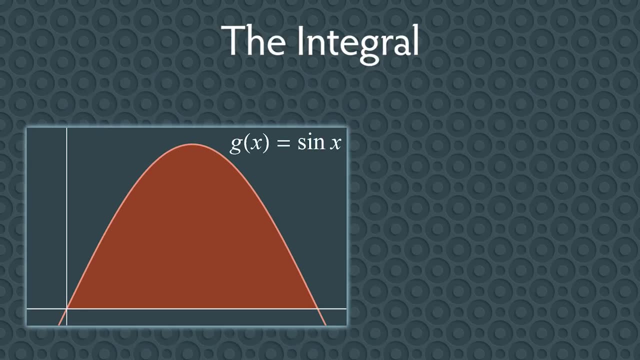 we do it. We know how to find the area of simple shapes like rectangles and circles, but this is much more curvy and complicated. Let's zoom in to get a closer look. Here is the idea: Slice the region into a bunch of very thin sections. Let's start with thin slices For each. 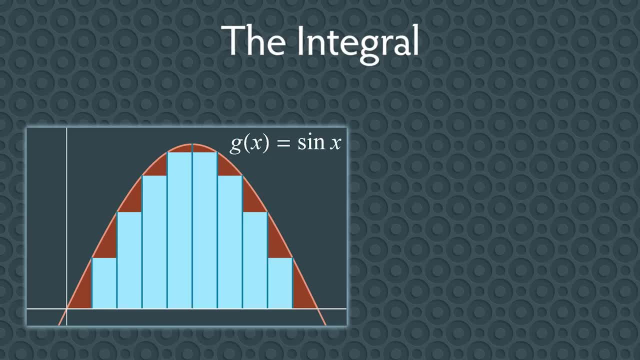 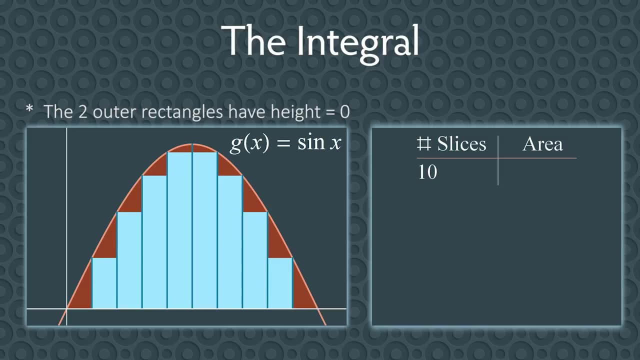 section, find the area of the tallest rectangle you can fit inside. There are 10 thin rectangles. The width of each rectangle is pi over 10, and we can find the height using the function g of x. Next, add up the areas of all 10 rectangles. We get a combined area of 1.66936.. This is a pretty 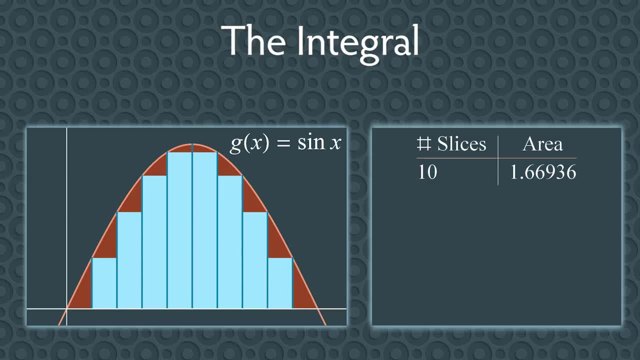 good approximation. Let's take a look at the area of the tallest rectangle. Here is the area of the shortest rectangle. We can't find the area of the tallest rectangle in any section, but we can do better. What if we do this again, but use 25 slices instead? This time we get an approximate area of. 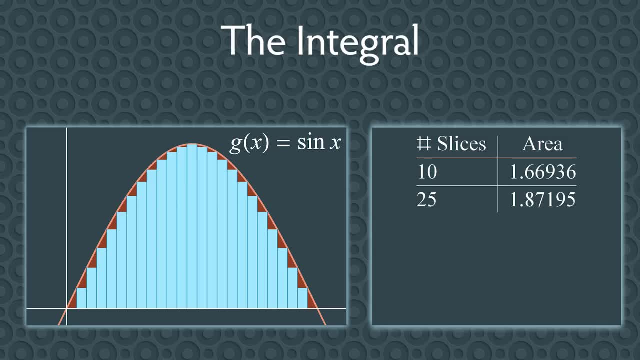 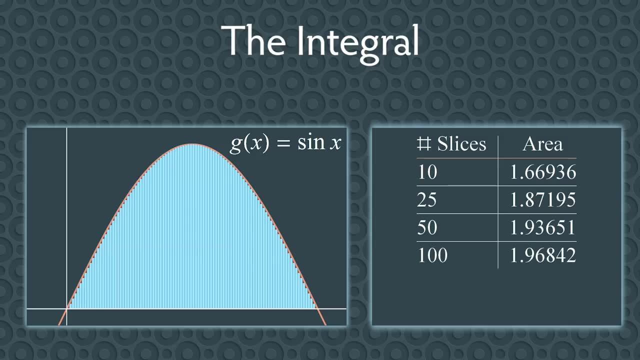 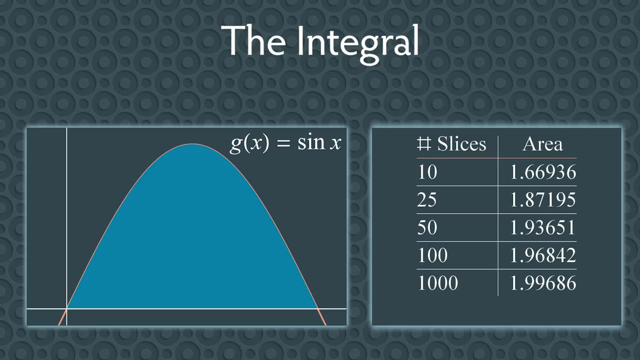 1.87195.. Let's do this again and again, using thinner and thinner slices- 50 slices, 100 slices, 1,000 slices- You get a sequence of areas that are getting closer and closer to some number. It looks like the area is approaching 20.. 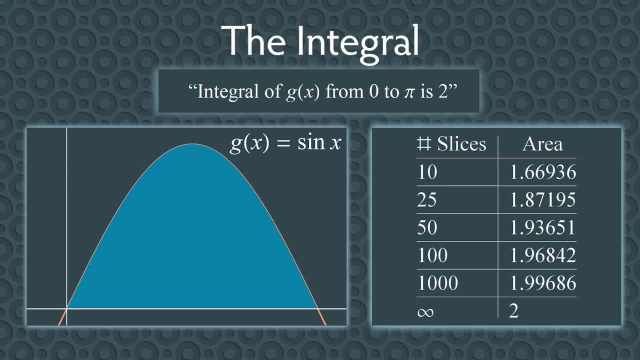 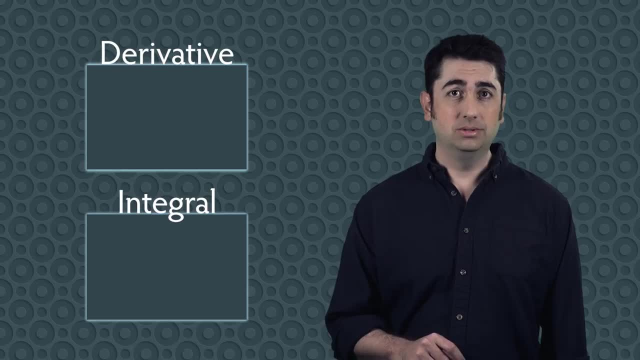 2. We call this area the integral of g of x, from x equals 0 to x equals pi. So we have these two tools: the derivative and the integral. The derivative tells us about a function at a specific point, while the integral combines the values of the function. 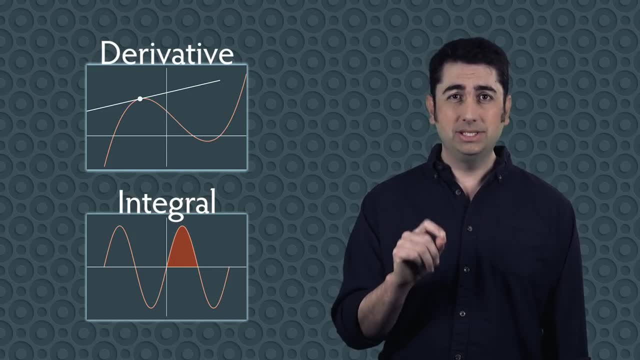 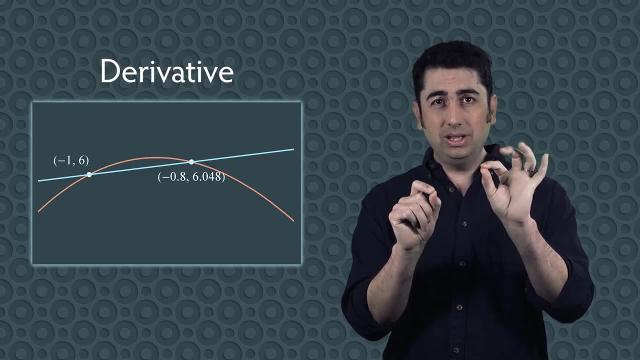 over a range of numbers. But notice, there is something similar to how we found the derivative and the integral. In the case of the derivative, we found two points that were close to each other. Then we let one point get closer and closer and closer to the point that we�re. 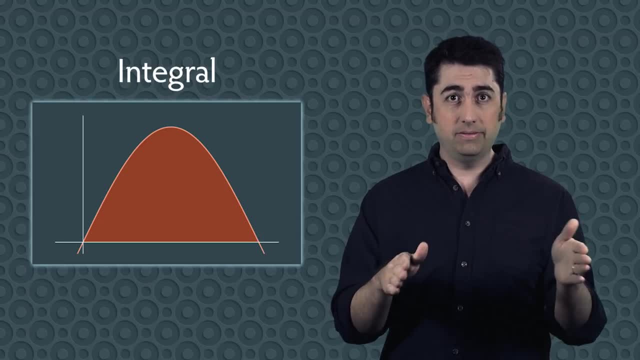 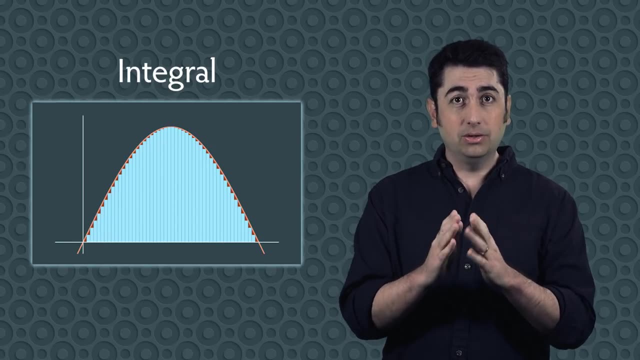 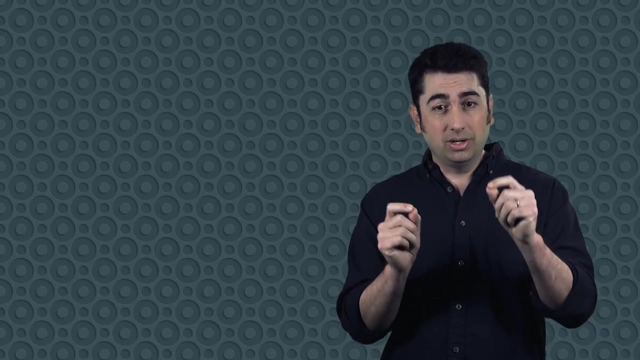 interested in. In the case of the integral, we took the curve and we chopped it up into a bunch of rectangles to approximate the area under the curve. Then we took thinner and thinner rectangles to get better and better approximations. In both cases we�re using the same technique. In the case of the derivative, we�re letting 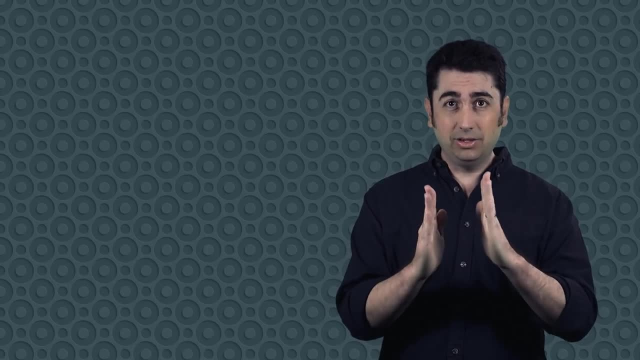 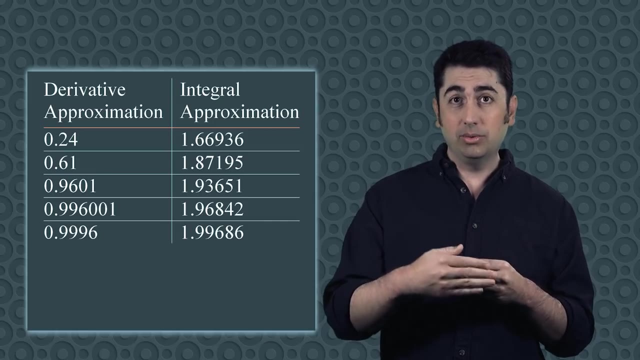 the points get closer to each other. In the case of the integral, we�re letting the rectangles get thinner. In both instances, we�re getting better and better approximations, better and better approximations, and we're looking at what number these approximations. 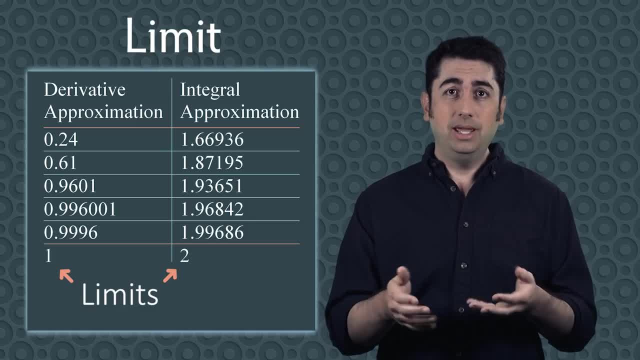 are approaching. The number they're approaching is called the limit, and because limits are key to computing both the derivative and the integral, when you learn calculus you usually start by learning about limits. A lot of your time in calculus will be spent computing derivatives and integrals. You'll 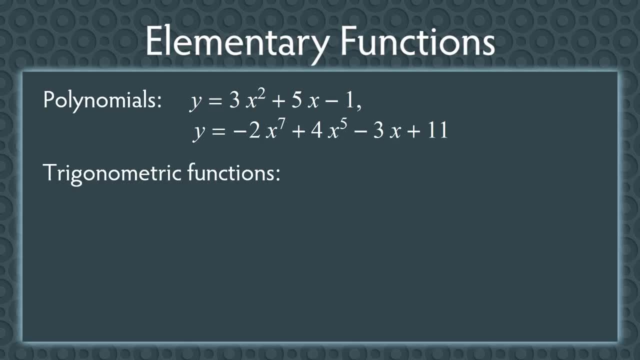 start with the essential functions: polynomials, trig functions, sine cosine and tangent exponential functions and logarithmic functions. These are the building blocks for most of the functions you'll work with. Next you'll make more complex functions by adding, subtracting. 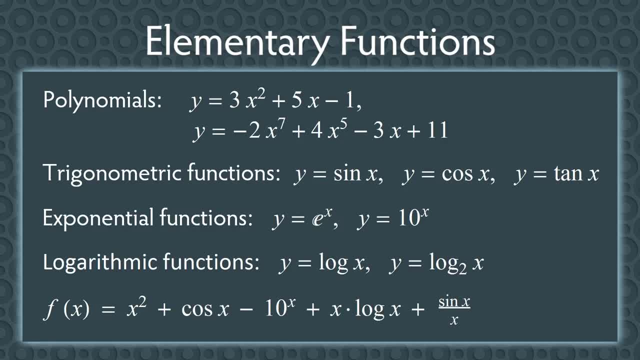 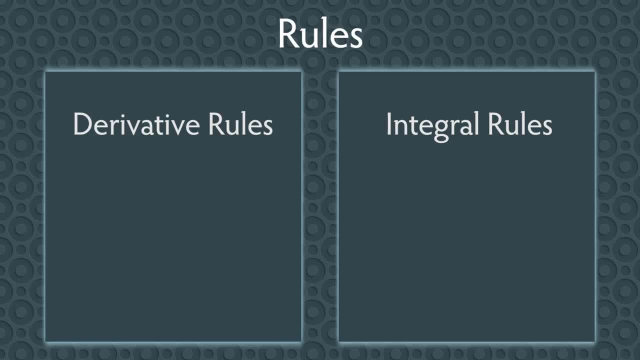 multiplying and dividing these functions together. You'll even combine them using function composition In calculus. there are a lot of rules to help you find derivatives and integrals of these more complex functions. The derivative rules have names like the product rule, quotient rule and chain rule. 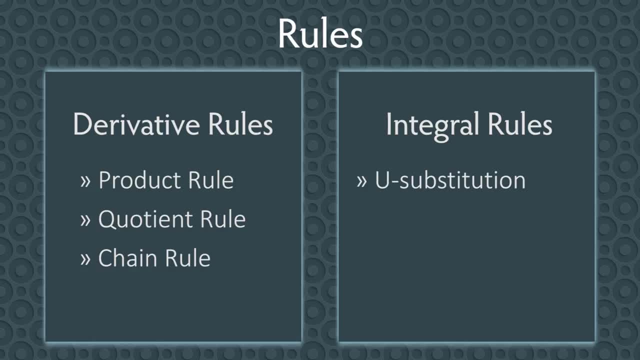 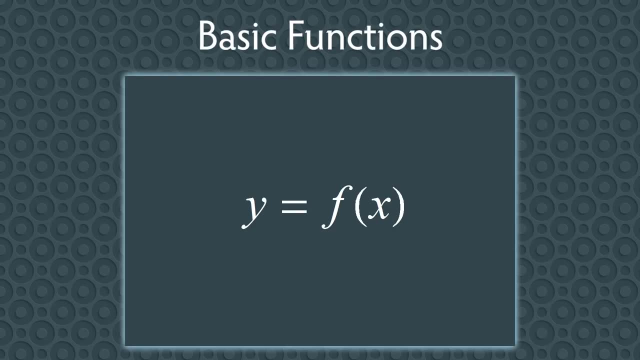 Subtitles by the Amaraorg community. The integral rules include u-substitution, integration by parts and partial fraction decomposition. When you first start calculus, your focus will be on basic functions, functions with one input and one output. But we don't live in a one-dimensional world. Our universe is 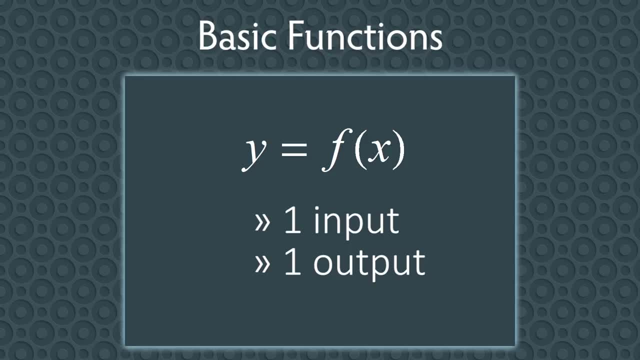 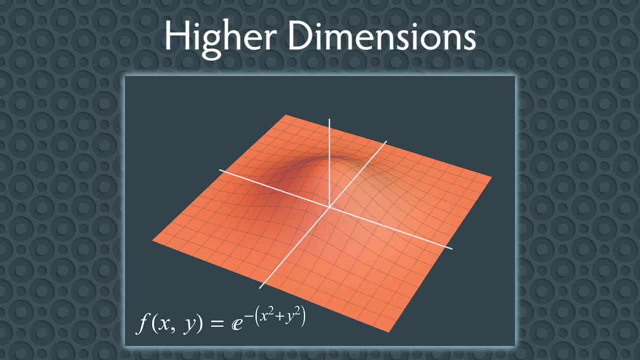 much more complicated. So once you've mastered calculus for basic functions, you'll then move up to higher dimensions. For example, consider a function with two inputs and one output like f. f equals e to the negative x2 plus y2.. Earlier we computed the derivative by computing. 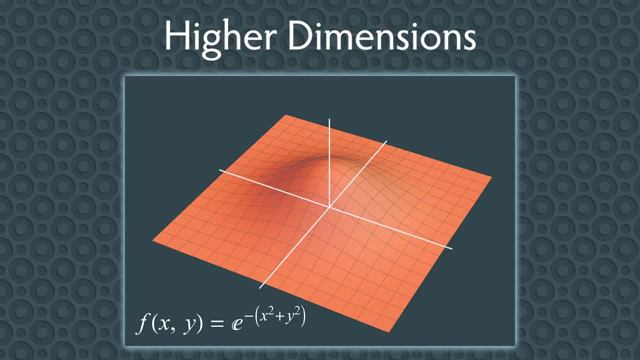 slopes of tangent lines. But in higher dimensions things are a bit more complex. This is because on a surface, instead of a tangent line you'll have a tangent plane To handle this. you'll compute the derivative both in the x-direction and in the y-direction. We call these partial. 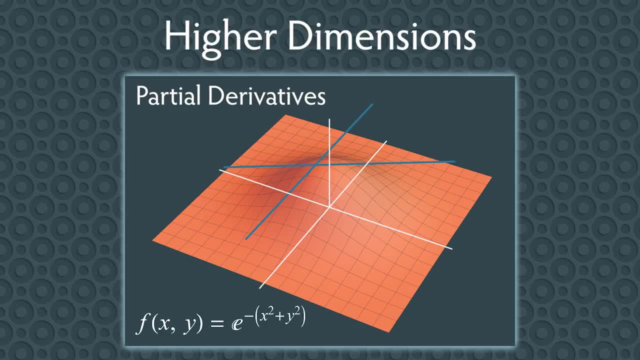 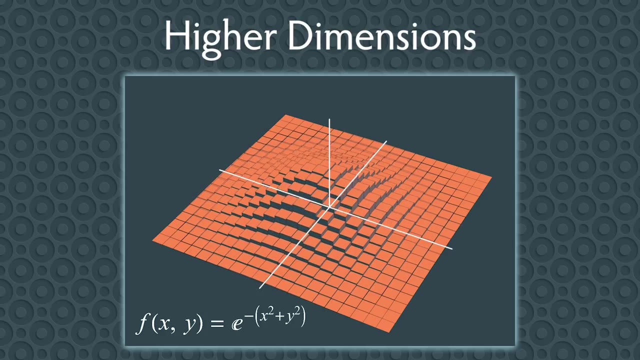 derivatives. These two partial derivatives are what you need to describe the tangent. We'll also need to generalize the integral. The region below a surface is three-dimensional. It has a volume, not an area To compute the volume. we'll approximate it using a bunch. 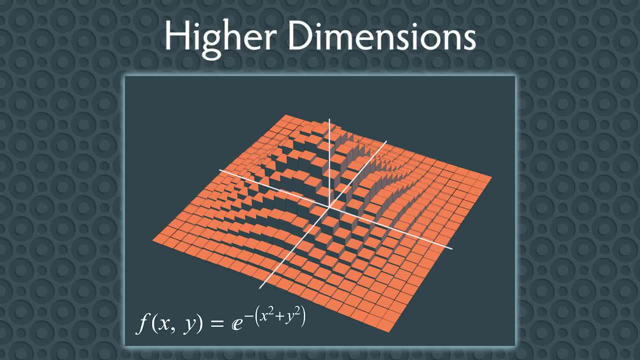 of skinny boxes. To sum up all the volumes, you'll need to use a double integral, because the boxes are spread out in two dimensions. But don't forget we live in three spatial dimensions, So you'll also need to learn calculus for functions with three inputs: x, y and 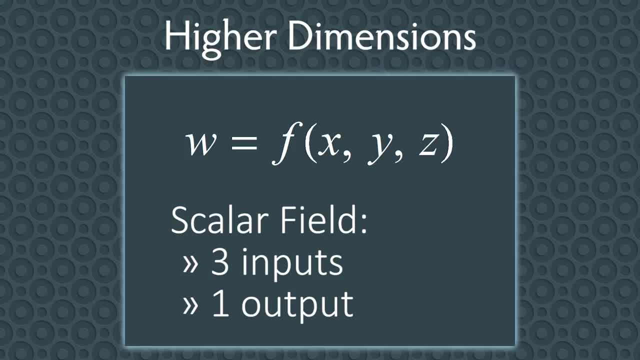 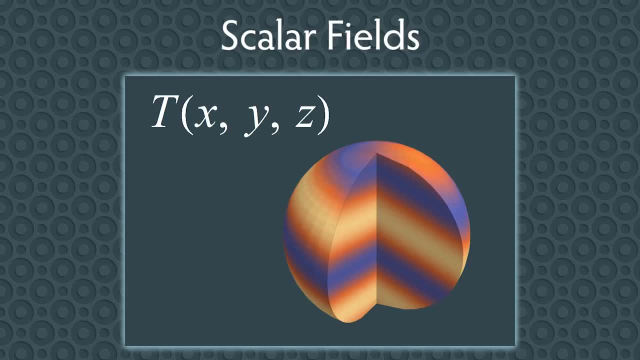 z. If a function has three inputs and one output, we call it a scalar field. An example would be a function returning the temperature at a given point in space. And the outputs of functions don't have to simply be numbers, They can also be vectors. A function with